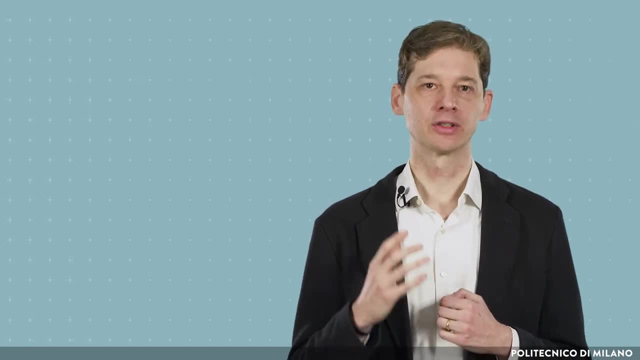 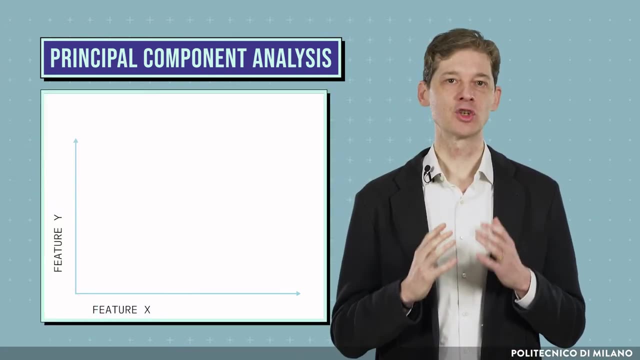 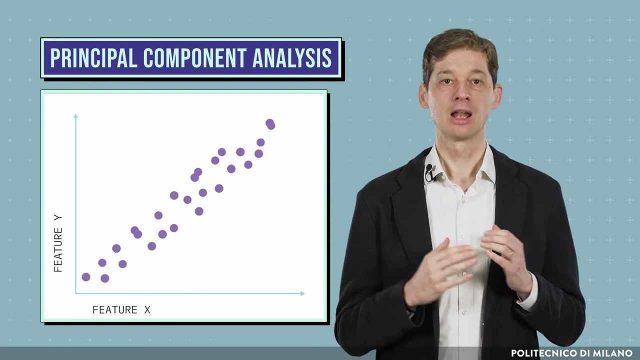 One of the most popular dimensionality reduction techniques is principal component analysis, or PCA. Starting from the original input features, PCA creates new features which are linear combinations of the original ones. Let's look at this image that shows points in a two-dimensional space. 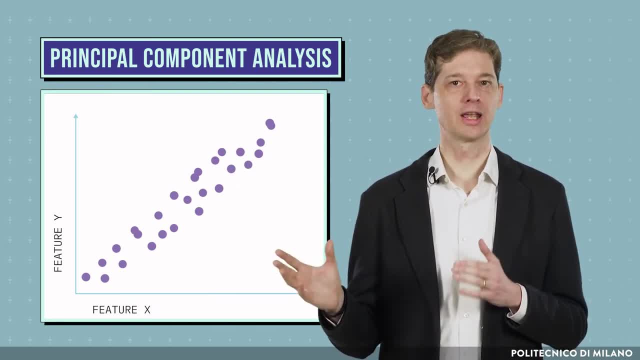 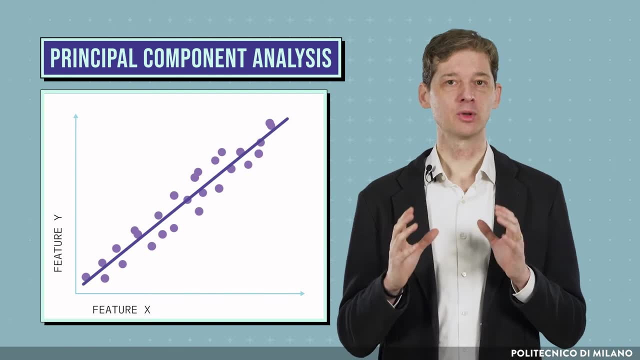 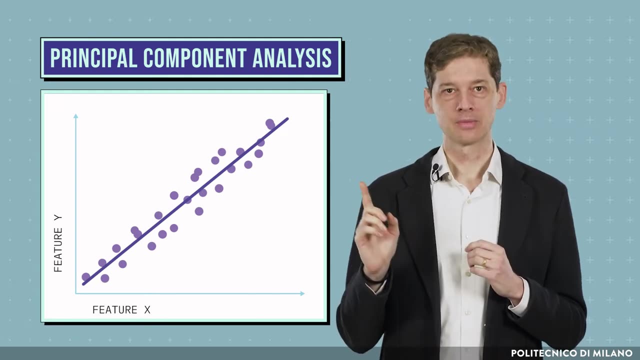 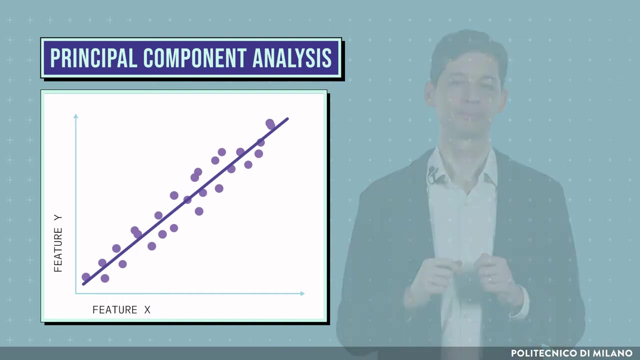 As we can see, these two features look very correlated with each other As the points lie very close to a line. If we want to reduce the input features from two to one, which choice would we make? If we consider that line and we project all the points onto that line, this will entail a linear transformation of our data. 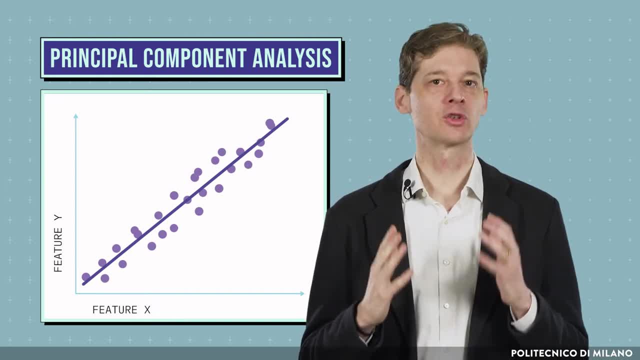 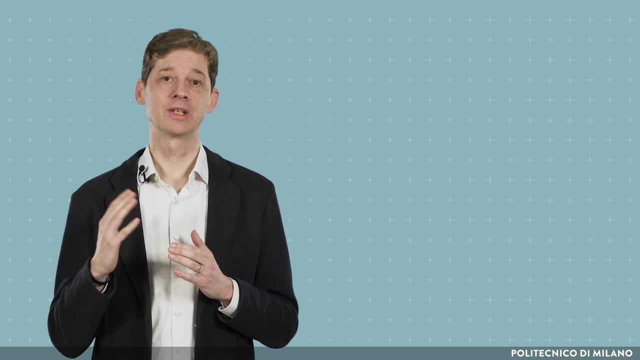 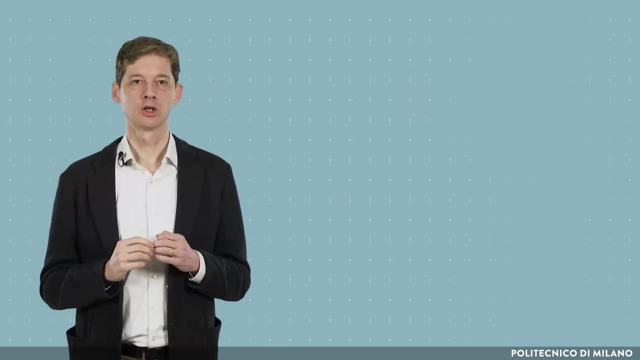 These new features allow us to replace the two original features by preserving the original information as much as possible. As we will see, the goal of PCA is to produce a new representation that retains the original variance as much as possible. So how does PCA find out these lines? onto which project in the data? 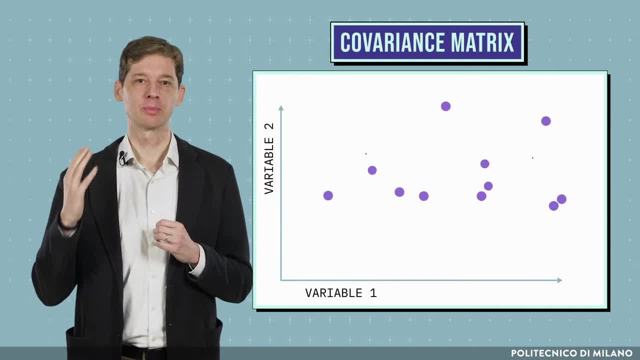 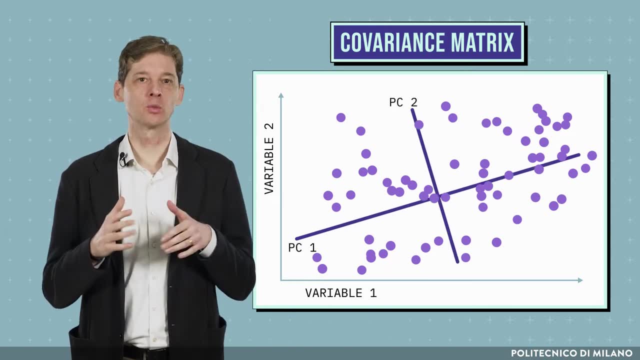 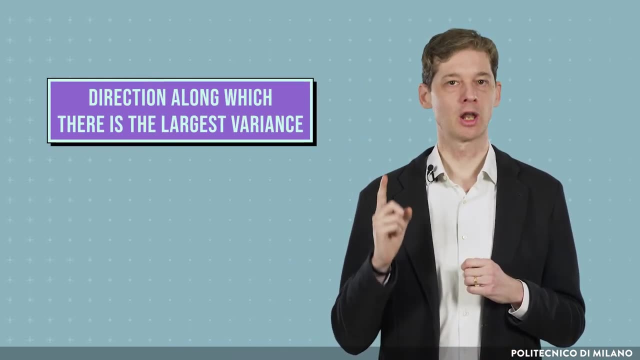 This is obtained by computing the covariance matrix of our dataset. Then, to know which is the most important direction, PCA considers the eigenvector associated with the largest eigenvalue. This is the first proof, This is the first principal component, that is, the direction along which there is the largest variance. 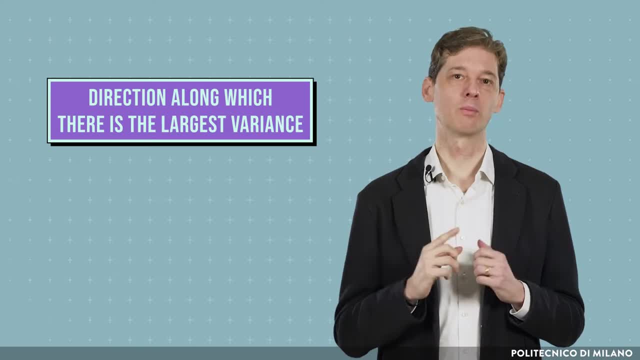 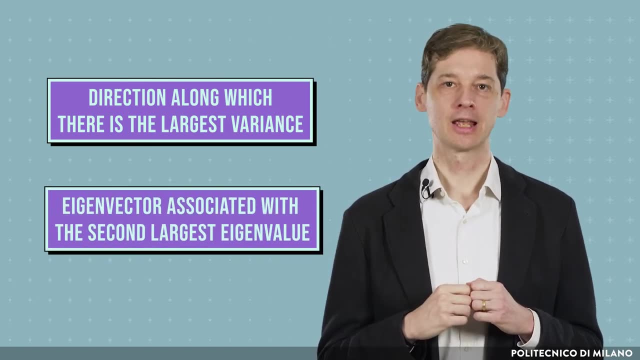 The values in the eigenvector specify the coefficients of the linear combination of the original input features. The second principal component will be the eigenvector associated with the second largest eigenvalue, and so on for all the other components. Given the properties of eigenvectors, all the new features are orthogonal to each other. 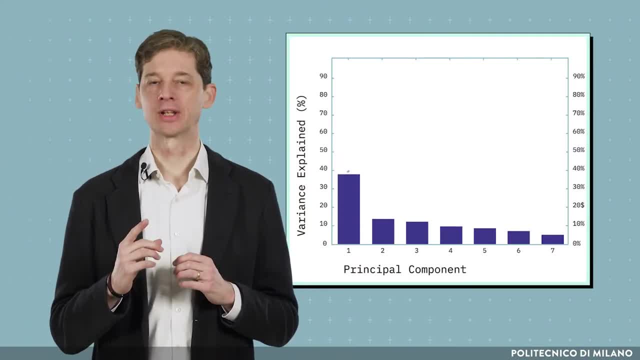 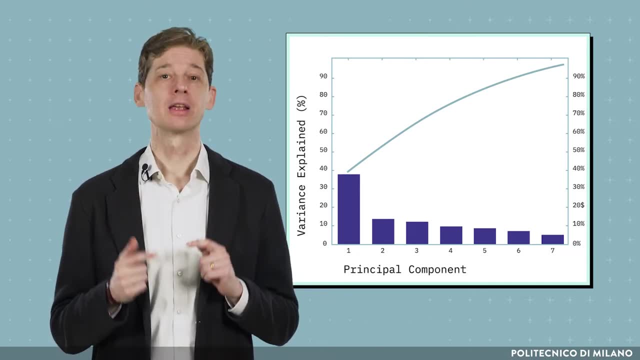 How can we choose how many and which principal components to select? First we must sort the eigenvectors in descending order of eigenvalue, Then given a threshold on the percentage of the original variance that we want to retain with the new representation. 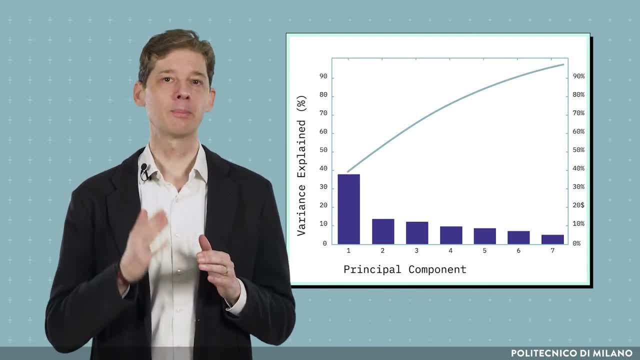 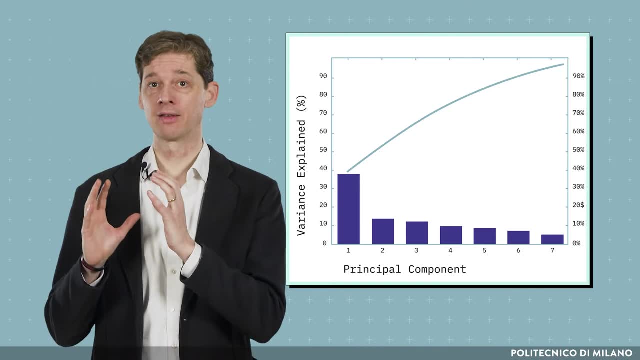 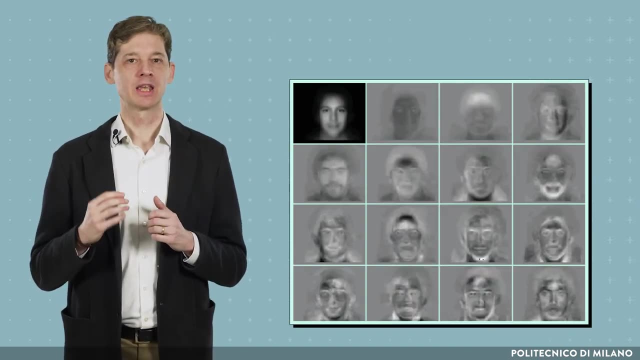 starting from the first principal component, we keep adding new features until the ratio between the sum of the eigenvalues of the selected components and the sum of the eigenvalues of all the components crosses the chosen threshold. In the picture we see an application of PCAs to a dataset of face images. 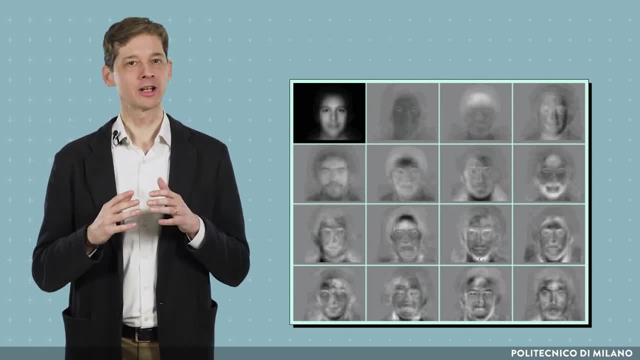 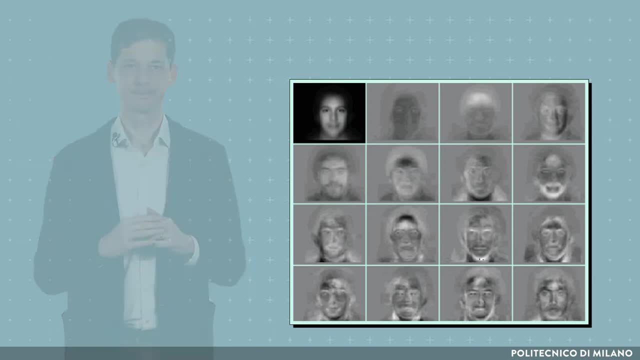 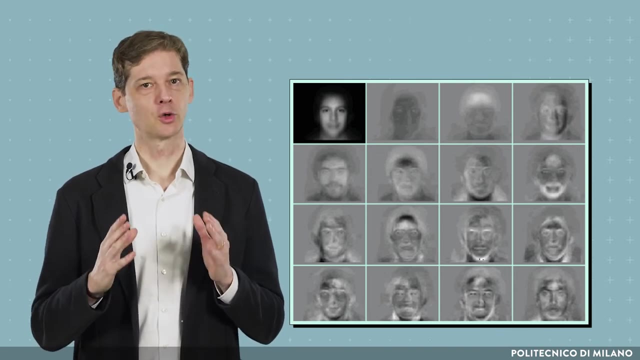 In the dataset there are 128 images of faces of size 256 times 128 pixels. In this picture we see a visual representation of the first 15 principal components, in this case called eigenfaces, And at the top left corner. 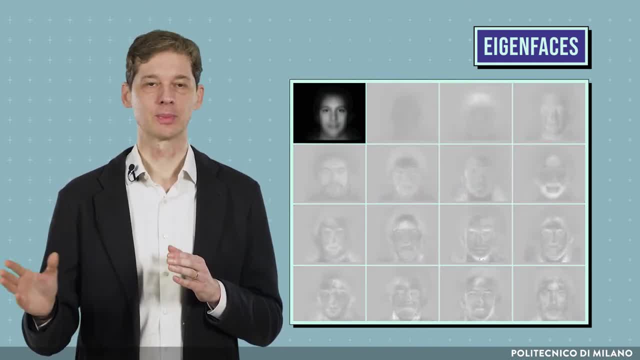 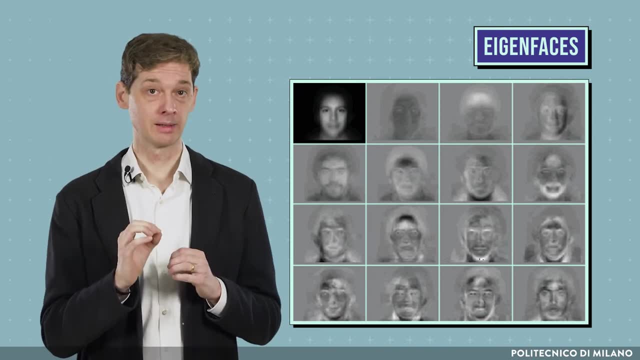 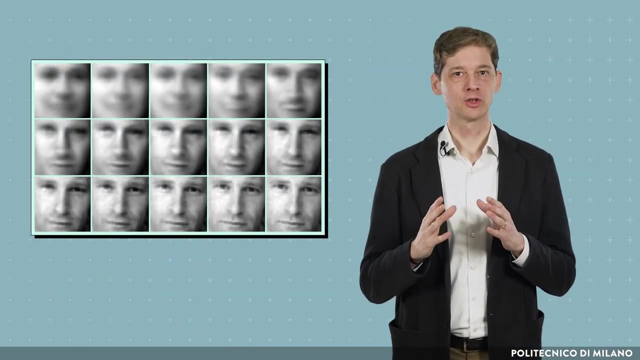 the reconstruction of a face in this 15-dimensional space. In this way, instead of using more than 30000 values to represent the intensity of each pixel, we can represent a face with only 15 values. Of course, as shown in this image, the accuracy of the reconstruction grows with the number of eigenfaces considered. 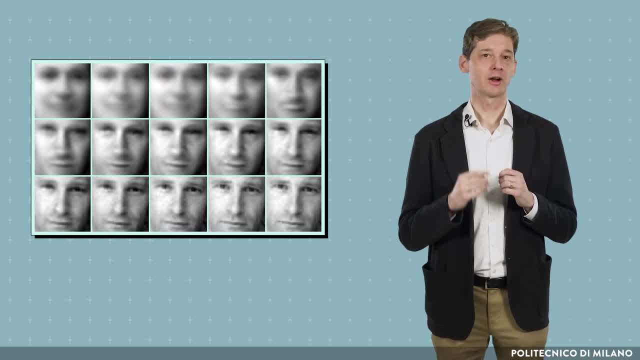 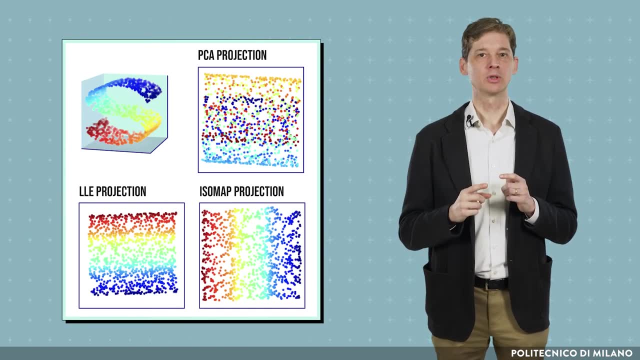 Unfortunately, linear combinations of the original features are not always able to capture the inherent structure in our data. If we have a dataset with examples distributed as in the picture, we will not be able to identify a principal direction, even if the data clearly occupies a manifold of the feature space. 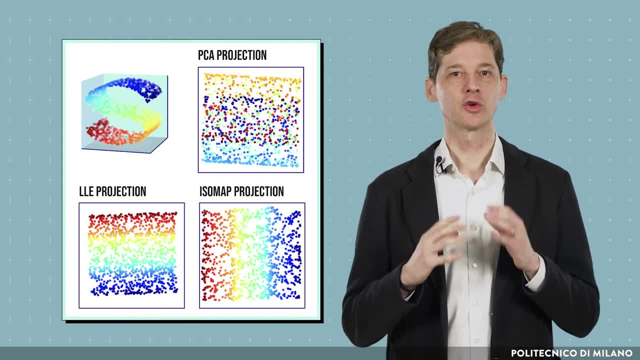 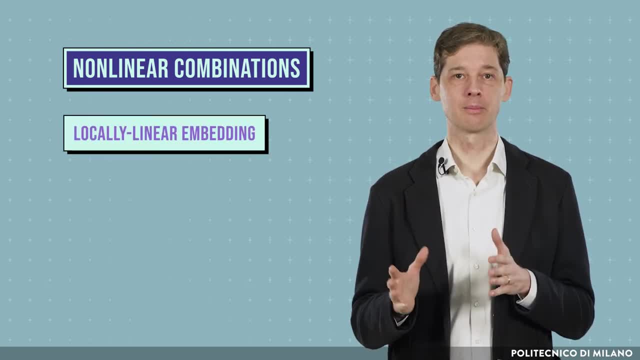 In this case, we need to resort to dimensionality reduction approaches able to create new features that are non-linear combinations of the original ones, such as locally linear, embedding, self-organizing maps, kernel, PCA, isomap and many others. 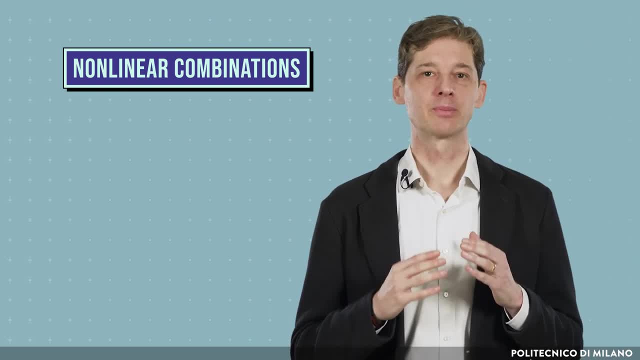 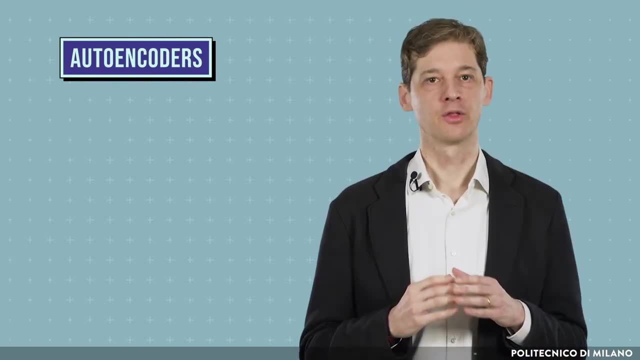 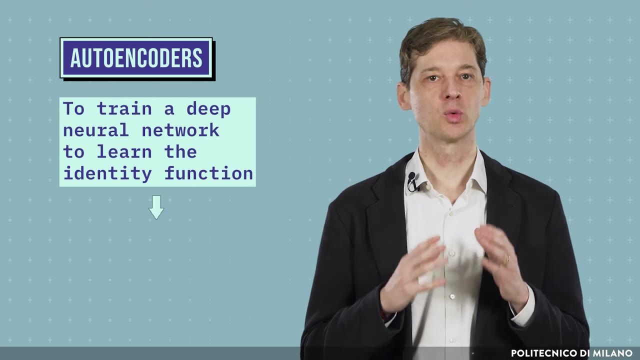 Recently also deep learning methods have been proposed to perform non-linear dimensionality reduction. A popular approach is called autoencoders. The idea of autoencoders is to train a deep neural network to learn the identity function. We want the network to be able to reproduce the input correctly.